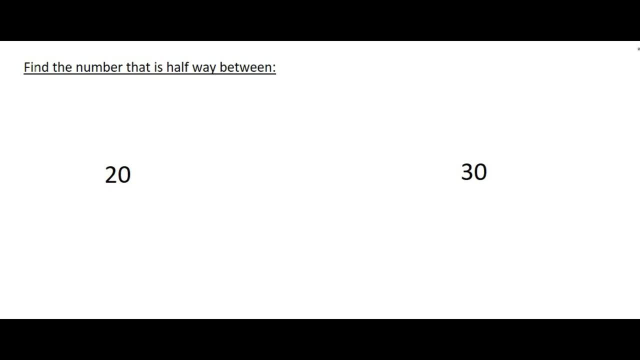 So we need to come up with a nice formula that can help us find the answer straight away. Many people I ask this question to they decide to. they tell me: well, maybe we can minus the two numbers together. well, minus the two numbers from each other, and then divide by two. 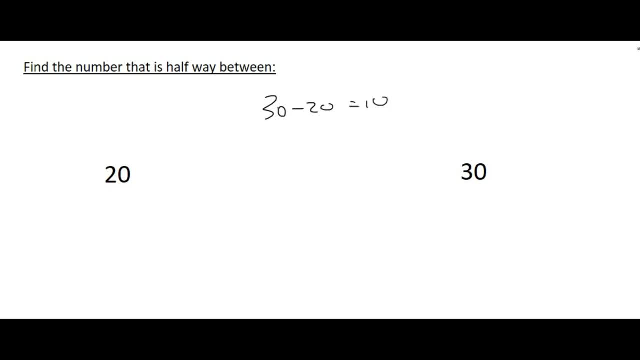 So 30 minus 20 is 10.. And then, if we divide that by two, we get five. And then they say: oh yes, well then we can just add that to the 20.. That isn't wrong, but it's quite a long method. 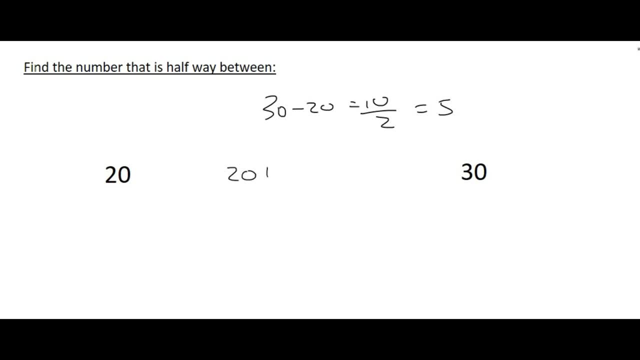 Let's go straight to the answer by adding the two numbers together and then divide that by two. Well, 20 plus 30 is 50. Divide that by two and you get 25.. So that is how you work out the midpoint of two numbers. 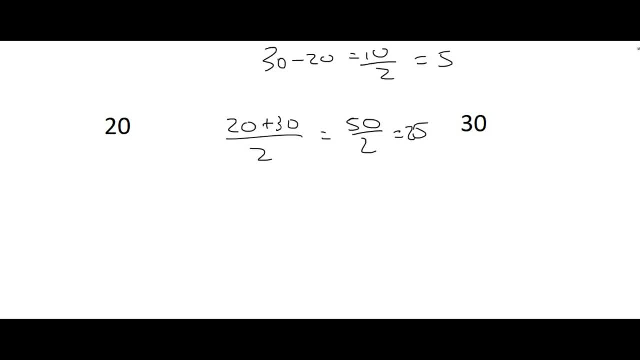 You add them together and you divide by two. So if I had to give you a set of coordinates like this and I asked you what is the coordinates exactly halfway between, Well, what you would do is you would do the X values by themselves. 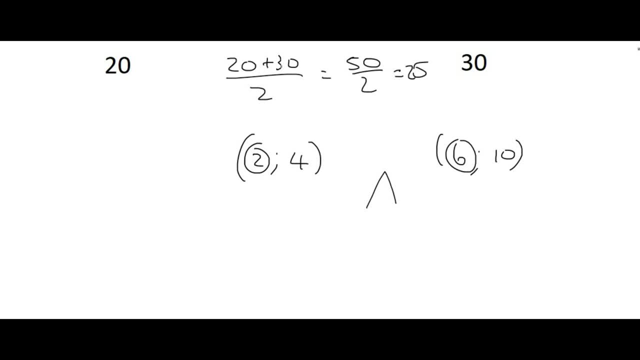 So you would add those together, which is eight, and then you would divide that by two, And that would give you four, And then you would do the Y values by themselves, And that would be four plus 10, which is 14.. And 14 divided by two is seven. 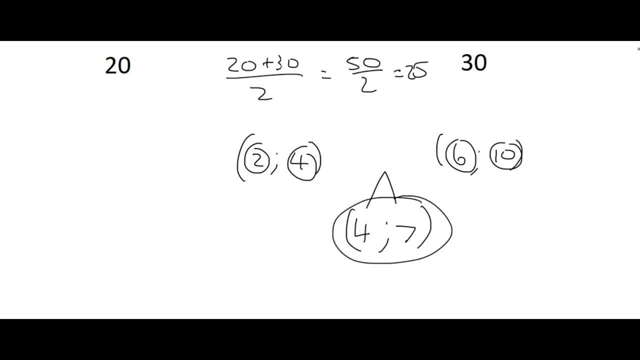 And so this would be the X value And this would be the midpoint of between those two points. So the midpoint is the halfway point between two points. So mathematically, the way we can work it out is as follows: And so here we have the midpoint formula. 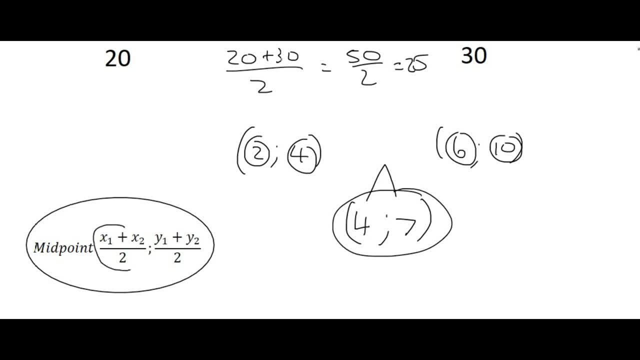 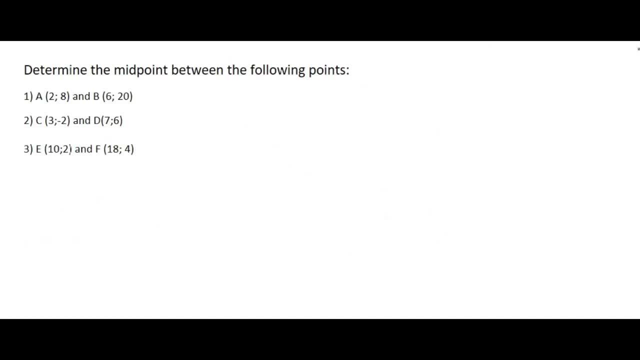 which says that you have to take the X values, add them together and divide by two, and then take the Y values, add them together and divide by two, And so let's work out the midpoint for each of these. So for number one, we're going to look at the midpoint between A and B. 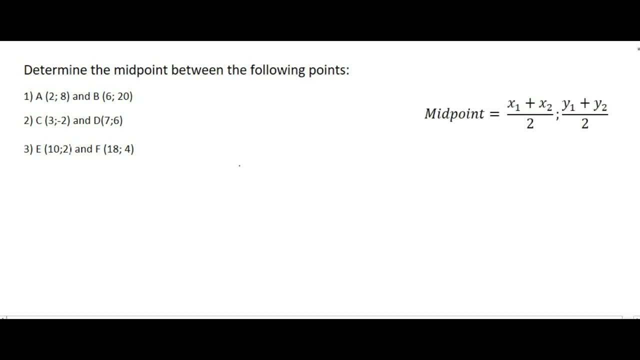 And so we're going to use the midpoint formula, And so we can, and so the mathematical way to do it is to say capital M, whereas if it was gradient you would use a small m. So we're going to say capital M of AB. 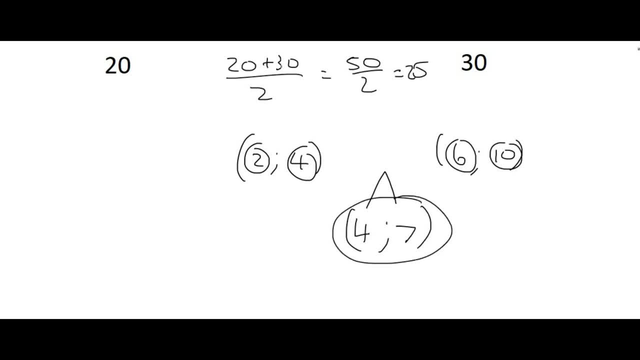 And so this would be 4 plus 10.. And this would be the midpoint of between those two points. So the midpoint is the halfway point between two points. So mathematically, the way we can work it out is as follows: And so here we have the midpoint formula, which says that you have to take the X values. 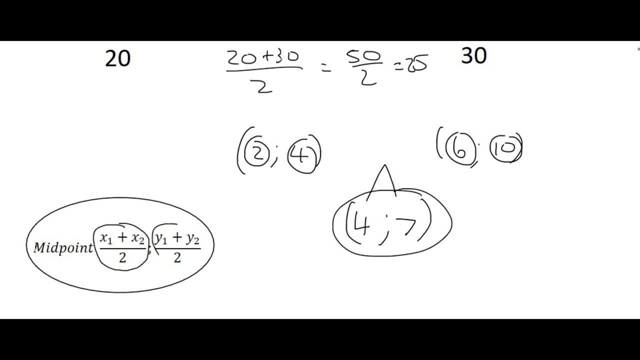 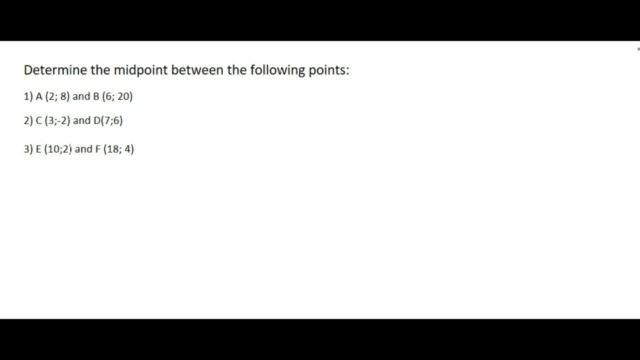 add them together and divide by 2, and then take the Y values, add them together and divide by 2.. And so let's work out the midpoint for each of these. For number 1, we're going to look at the midpoint between A and B. 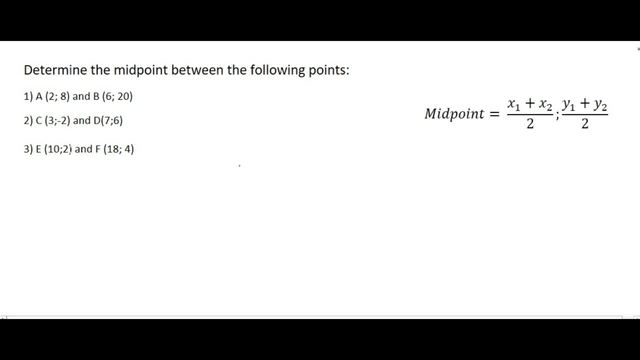 And so we're going to use the midpoint formula, And so the mathematical way to do this is to say capital M, whereas if it was gradient you would use a small m. So we're going to say capital M of AB. I'm going to call this point 1 and I'm going to call this point 2: equals. 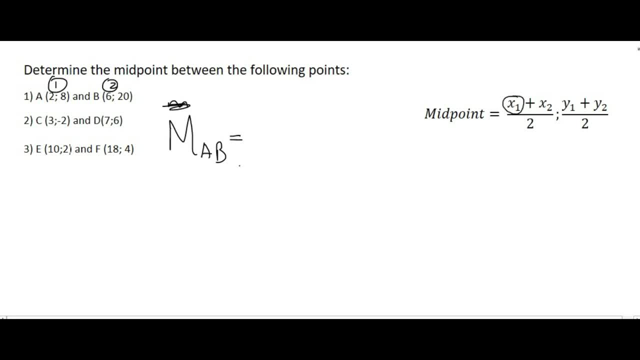 The formula says that we should take the X value of point number 1.. Well, that's going to be equal to 2 plus the X value of point number 2, which is the same. So we're going to take the Y value of point number 1, which is 6, and we're going to divide that by 2.. 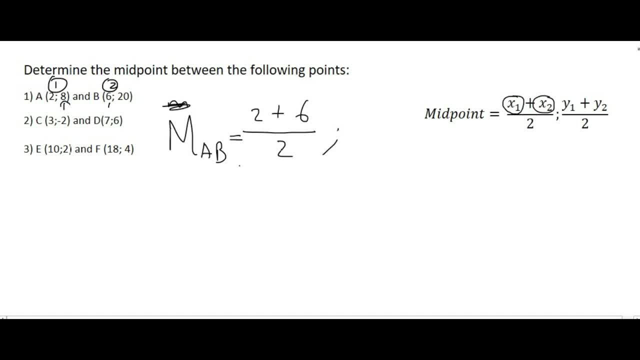 Then we're going to do the Y values. So we take the Y value of point number 1,, which is 8, and we plus the Y value of point number 2,, which is 20, and we divide by 2.. 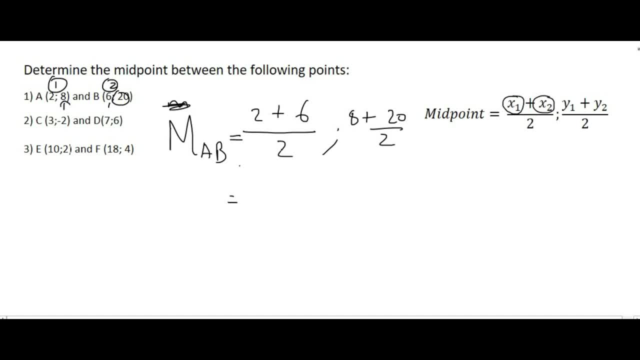 Then we do each part separately. So 2 plus 6 is 8.. 8 divided by 2 is 4.. And 8 plus 20 is 28.. And 28 divided by 2 is 14.. And so the midpoint of those two points, the midpoint of AB, will be 4.. 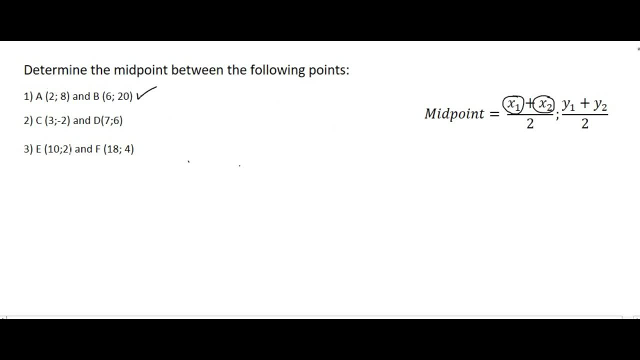 4 and 14.. Moving on to the midpoint of CD, where I'll call C, point number 1, and D, point number 2.. And then I'll just use the formula, So the X value of 1 is 3 and the X value of 2 is 7.. 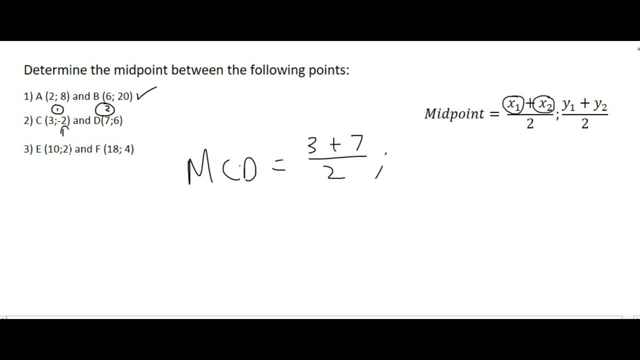 I'm then going to do the Y values. So the Y value of 1 is minus 2 and the Y value of 2 is 6 over 2.. So then, 3 plus 7 is 10.. 10 divided by 2 is 5.. 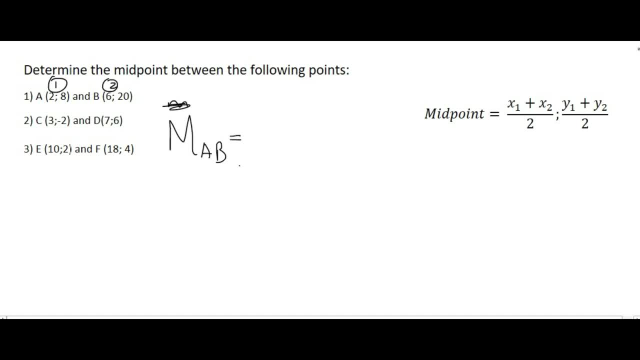 I'm going to call this point one and I'm going to call this point two- equals. The formula says that we should take the X value of point number one. Well, that's going to be equal to two plus the X value of point number two. 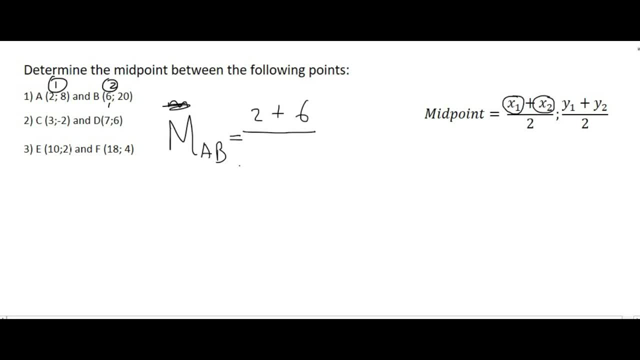 which is the six, and we're going to divide that by by two. Then we're going to do the Y values. So we take the Y value of point number one, which is eight, and we plus the Y value of point number two. 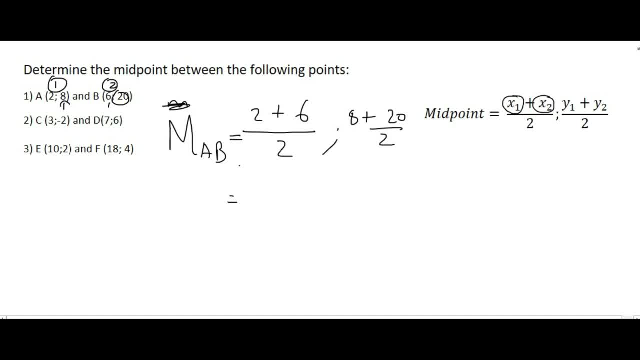 which is 20, and we divide by two, then we do each part separately. So two plus six is eight. eight divided by two is four, and eight plus 20 is twenty eight, and twenty eight divided by two is 14.. And so the midpoint of those two points. 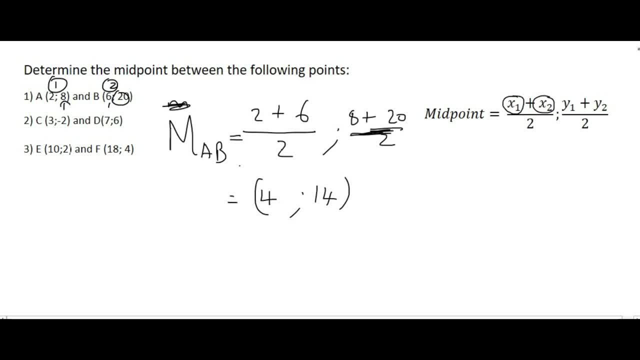 but the midpoint of AB will be four and 14. moving on to the midpoint of CD, We are called C, point number one, and D, point number two, and then I'll just use the formula. so the X value of one is three and the X value of two is seven, and then going to do the Y values. 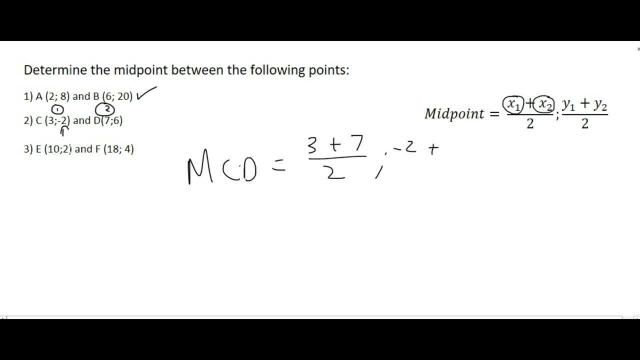 So the Y value of one is minus two and the Y value of two is six over two. So then three plus seven is ten. ten divided by two is five minus two plus six is four. four divided by two is two, And there's the answer for that. 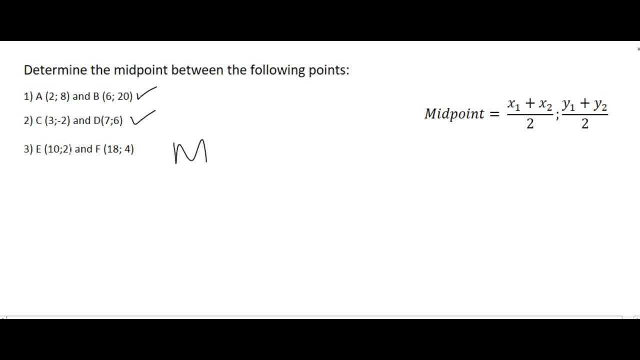 And finally, moving on to the midpoint of EF. so we'll go capital M EF. I'm going to call E's point number one and F point number two. So the formula says that I must take the X value of point number one. 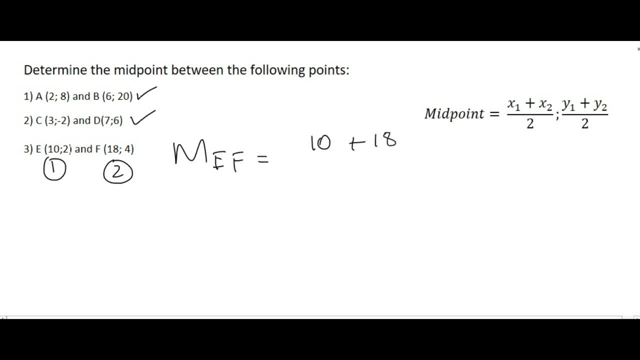 That's going to be ten, plus the X value of point number two, which is 18, and I'm going to divide that by two. Then I'm going to take the Y value of point number one, which is two, Then the Y plus the Y value of point number two, which is four, and divide that by two. 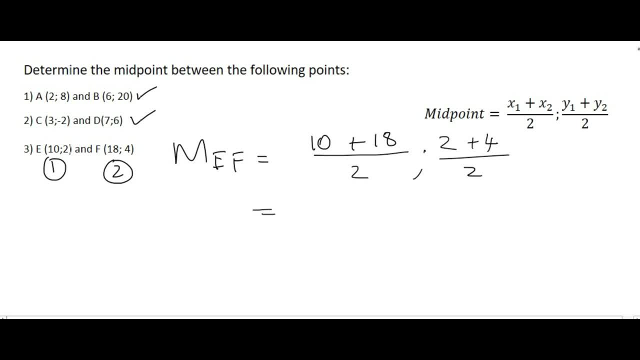 So ten plus 18 is twenty eight. twenty eight divided by two is fourteen. Two plus four is six. six divided by two is three, And so the midpoint of EF is fourteen and three.